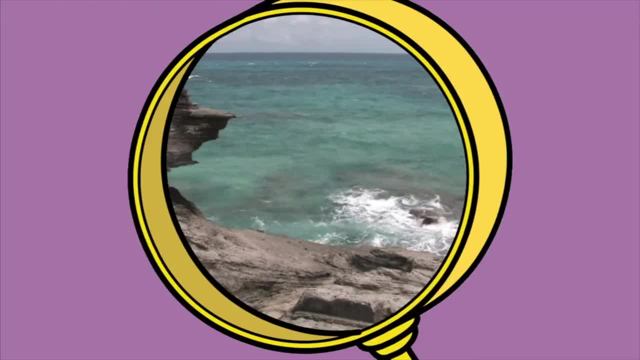 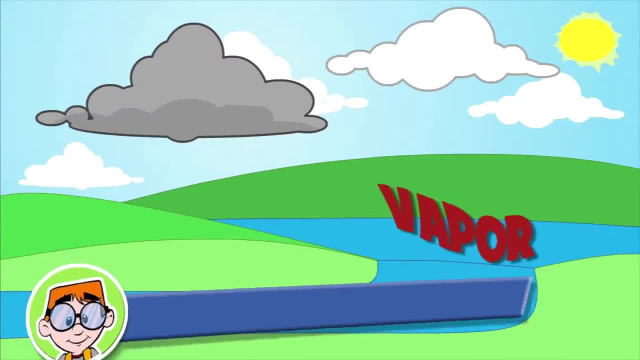 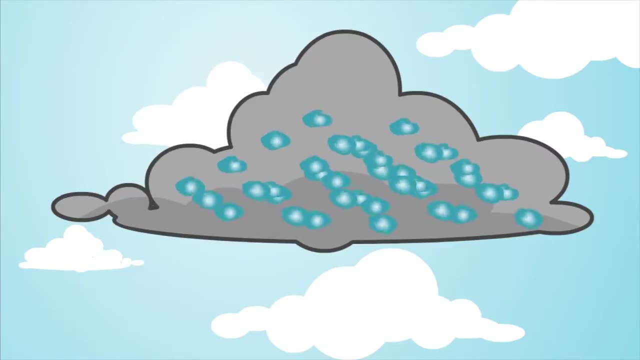 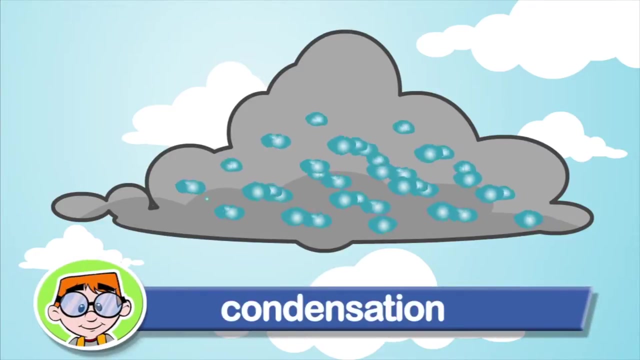 The sun heats a body of water like the ocean. The water evaporates or turns into steam or vapor and then travels up into the sky. Then the water vapors become cooler and come together, collecting in clouds. It's called condensation. 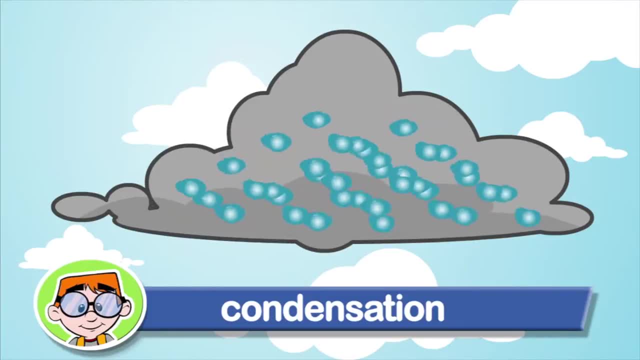 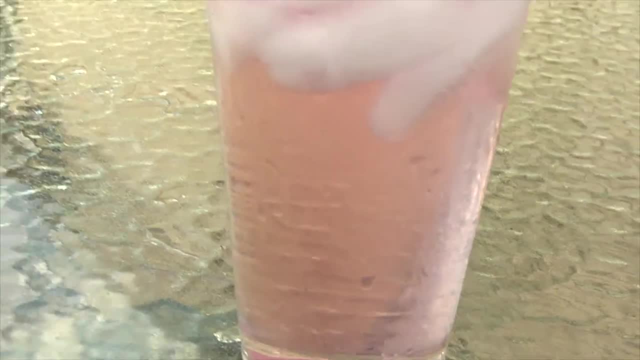 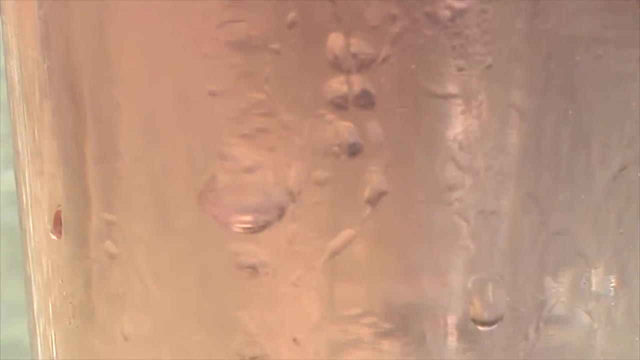 Here's an example of condensation. When you pour a glass of cold water on a hot day, you'll notice that water forms on the outside of the glass. The water on the outside of the glass came from the air. Water vapor in the air turns back into a liquid when it touches the cold glass. 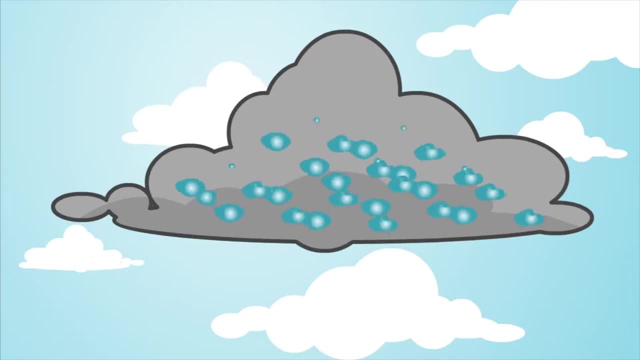 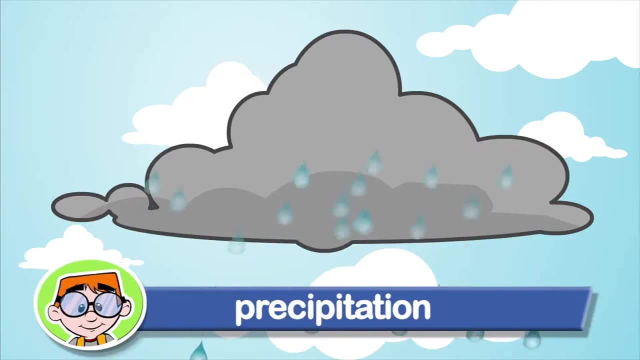 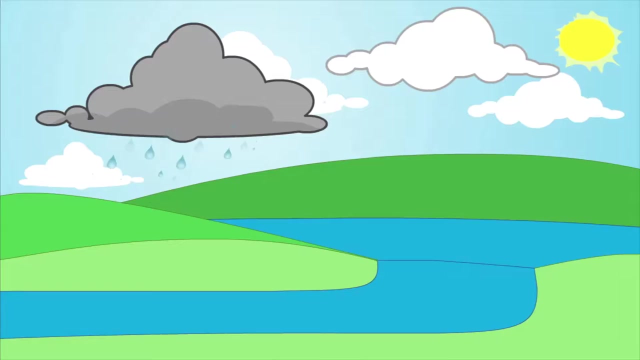 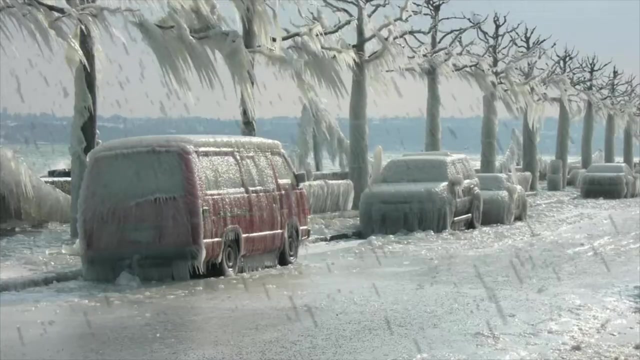 That's condensation. If there's enough water in the clouds, the water will fall to the earth. We call it precipitation. Precipitation happens when there is so much water packed together that the air can't hold it anymore. The clouds get heavy and water falls back to the earth as rain, hail, sleet or snow. 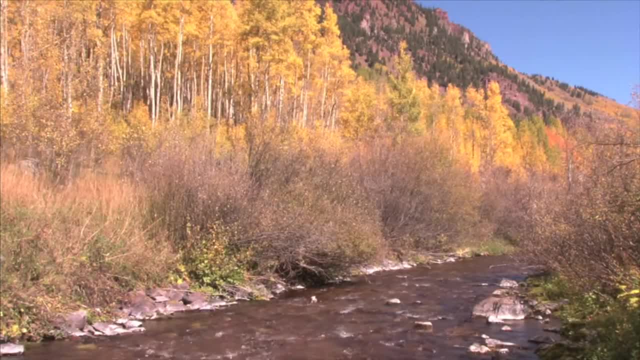 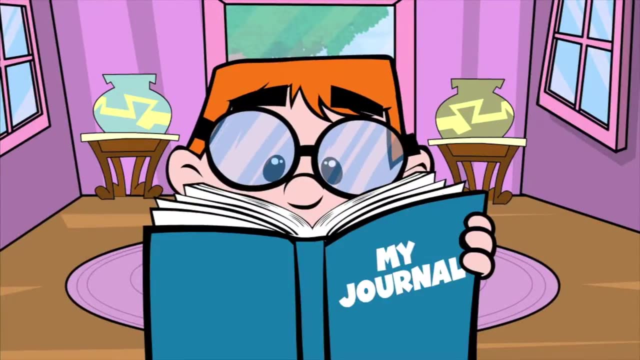 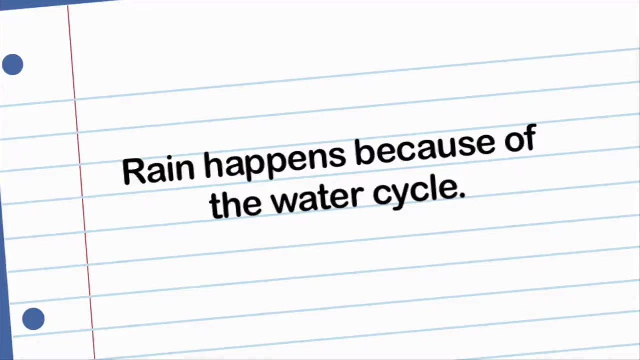 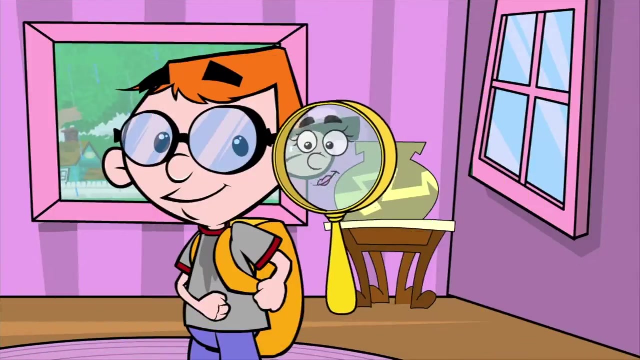 Some of the rain will collect in the ground to begin the water cycle all over again. I'm gonna write that down in my journal. Rain happens because of the water cycle. Got it Clouds? Can you tell us more about clouds Like, do all clouds carry rain? 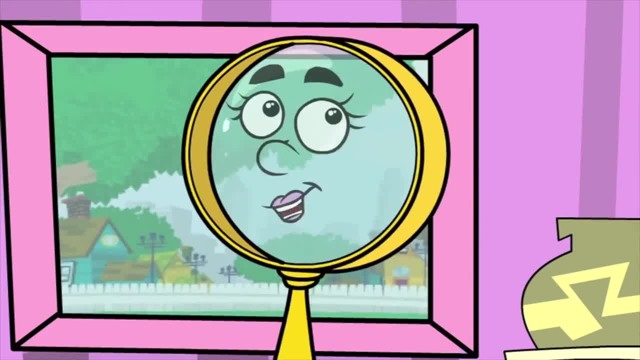 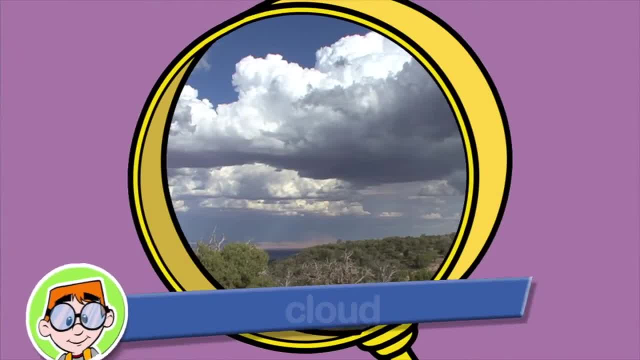 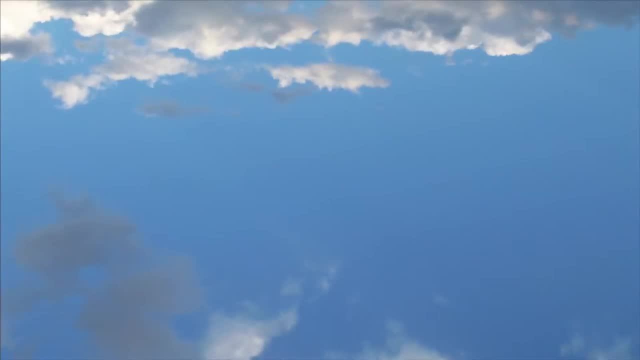 I was wondering the same thing. Excellent question, Here's the answer. A cloud is made up of very tiny droplets of water or ice crystals. The droplets are so small and light that they can float in the air. Clouds float in the earth's atmosphere. 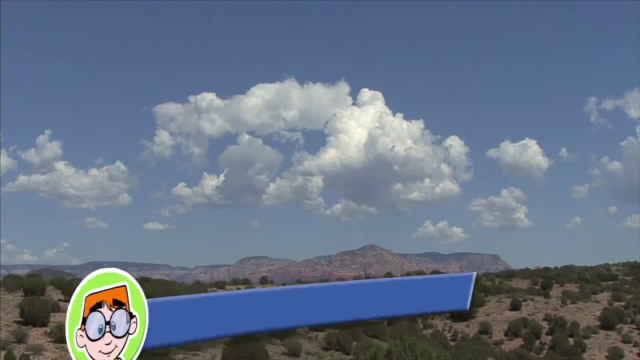 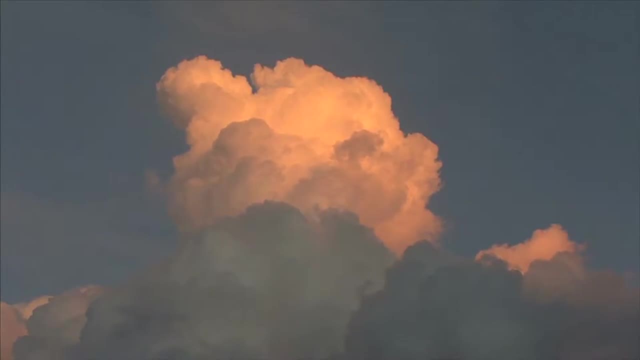 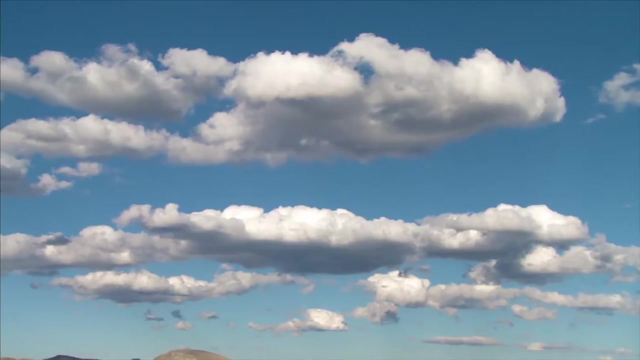 There are different kinds of clouds. Some clouds, called cumulus clouds, are puffy, white and appear in the sky on bright, sunshiny days. These clouds are white because they reflect the light of the sun. They are not rain clouds. 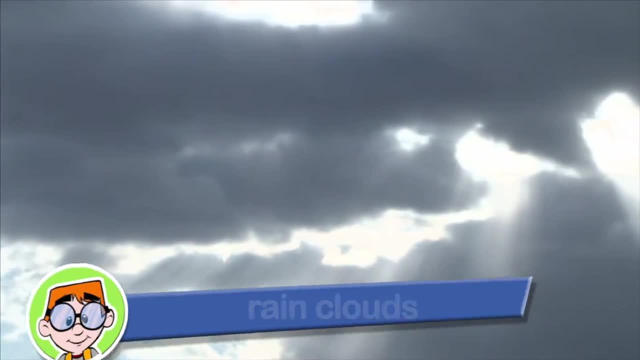 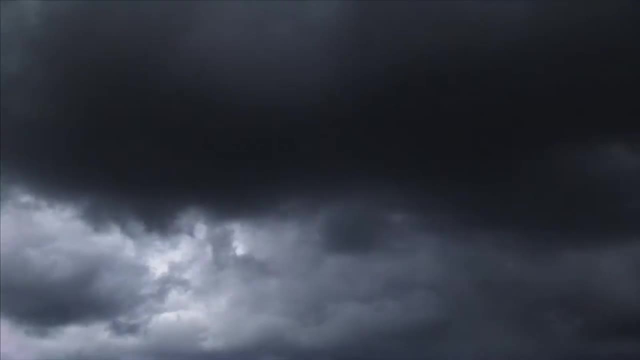 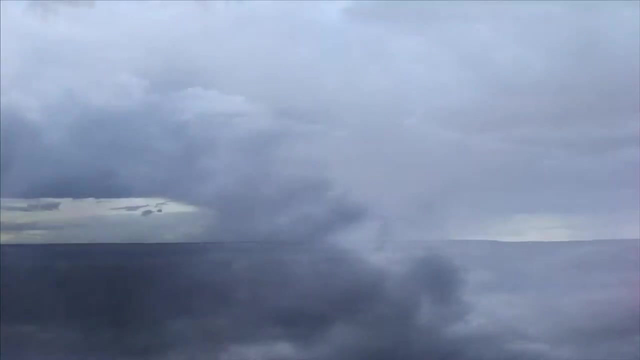 Then there are rain clouds. Rain clouds are caused by the buildup of water droplets or solid ice crystals. If these clouds get very thick or high in the sky, sunlight doesn't make it through. That's why rain clouds are grey. Nimbostratus clouds are the dark rain-carrying clouds. 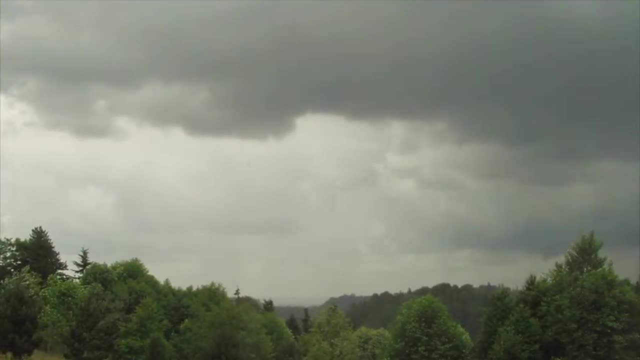 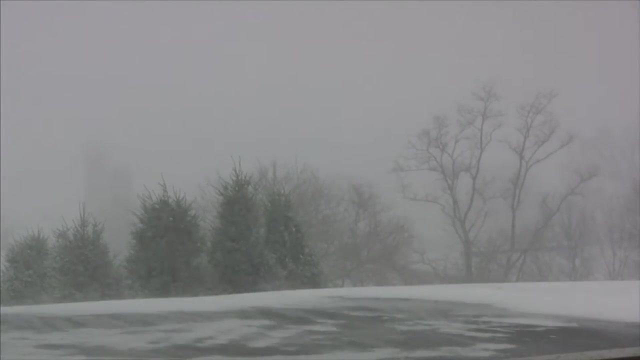 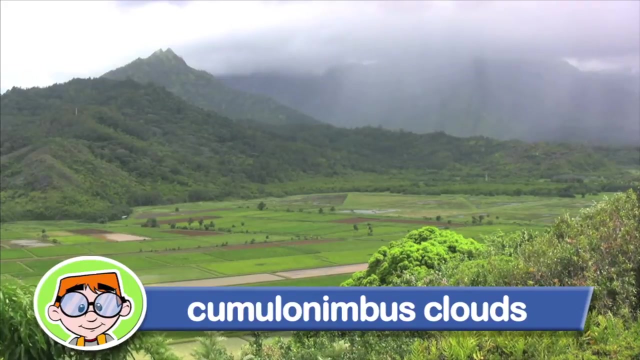 of bad weather. They can be found in both summer and winter, But they are mostly seen in the winter. These clouds cover the sky and block the sun. Cumulonimbus clouds produce showers and thunderstorms. The rain comes and goes with these clouds. 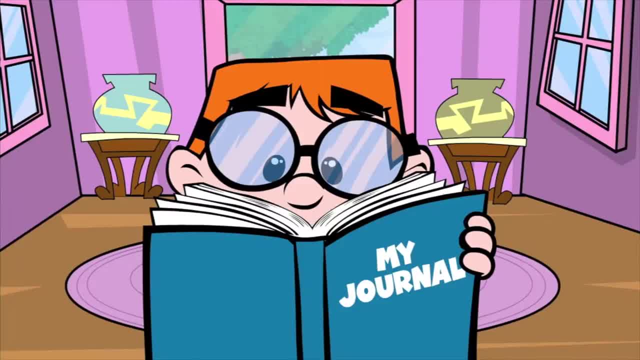 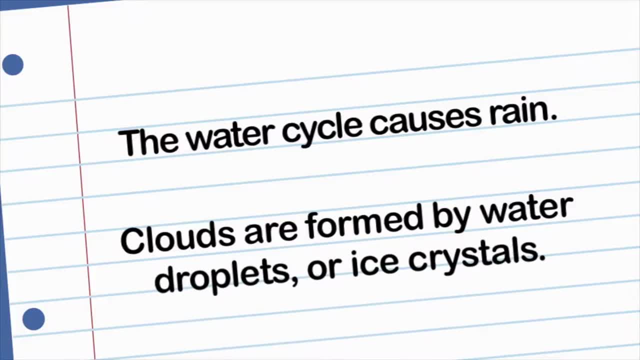 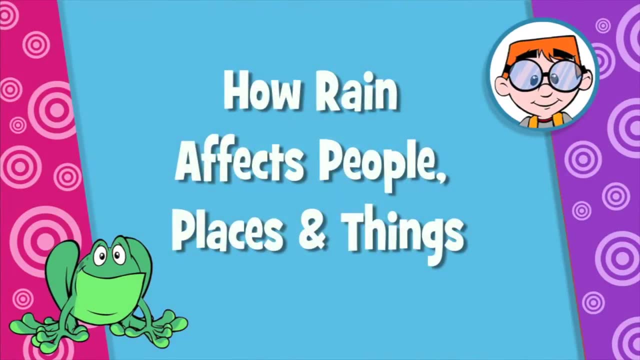 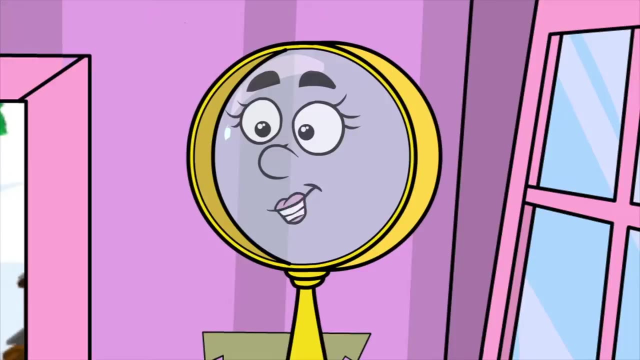 I get it. The water cycle causes rain And clouds are formed by water droplets or ice crystals. Got it How rain affects people, places and things? Rain, or the lack of rain, can really affect the land, plants, people and animals too. 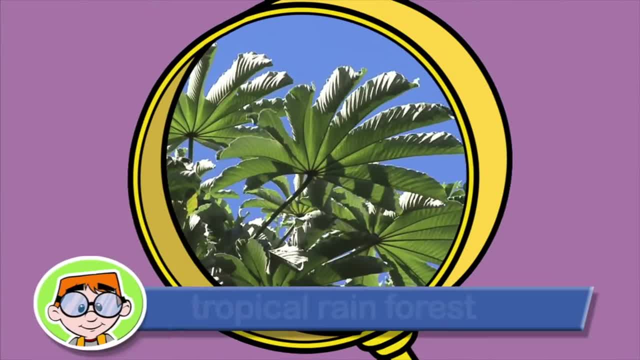 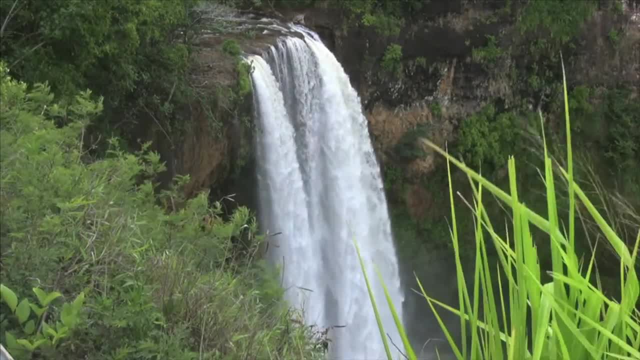 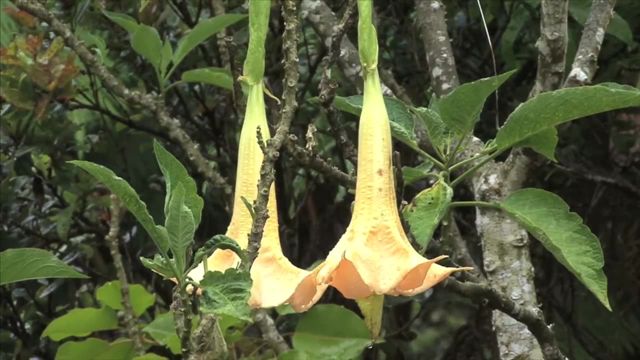 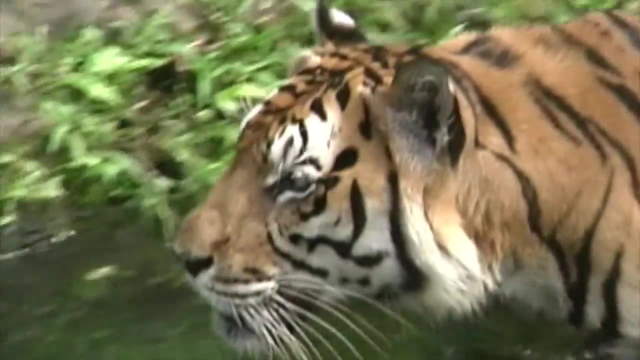 A place that gets lots of rain is a tropical rainforest. Because of the rain and an abundance of water, it makes the rainforest a great place to live for lots of animals and lots of plants. Rainforests are home to very strange and exotic plants and animals, both large and small. 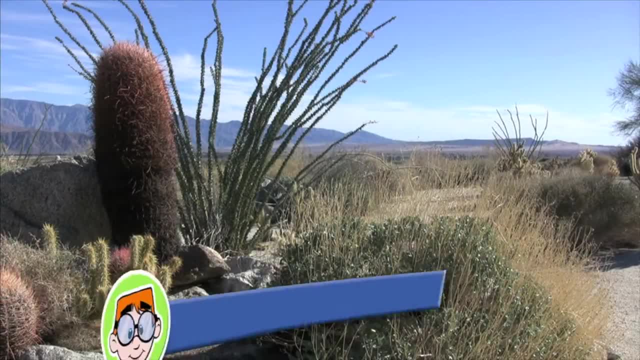 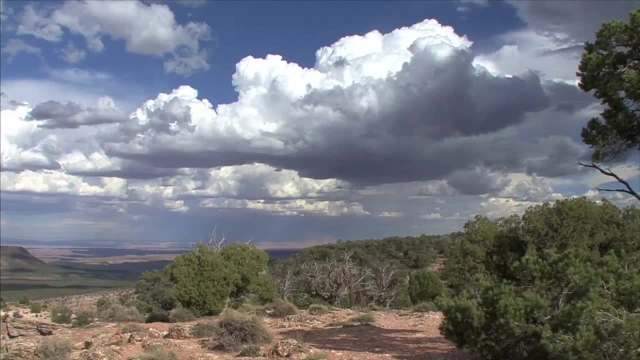 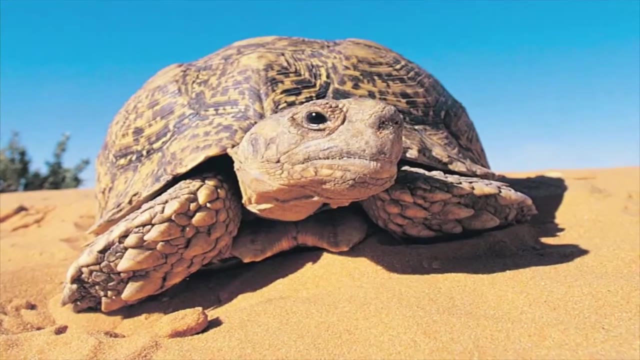 Some places on Earth do not receive a lot of rain at all. They are called deserts. Rain evaporates in the air before it hits the ground and dries. Because there is such little rain and a lack of water, not many plants or animals live in the desert. 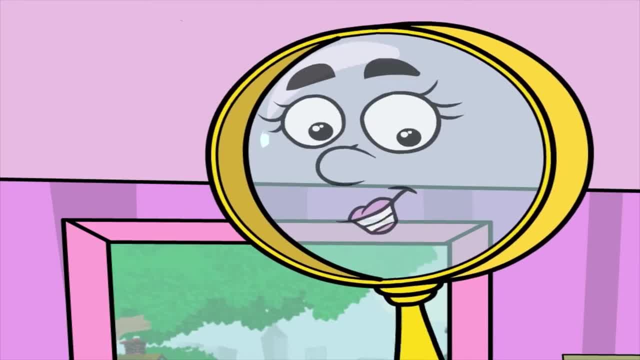 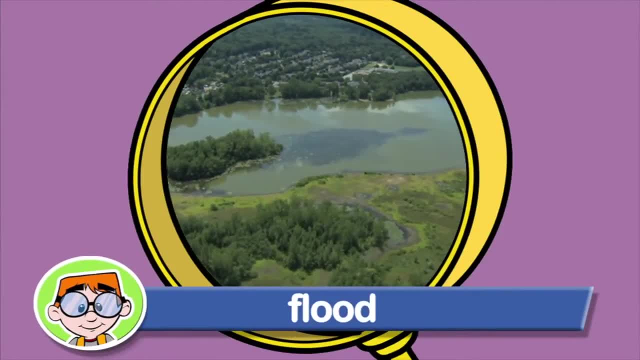 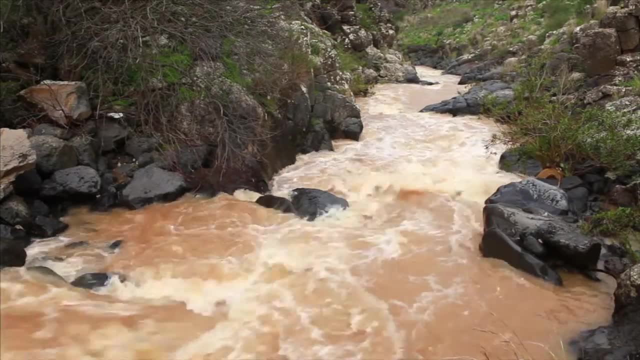 Can there ever be too much rain? Sometimes having too much rain can cause a flood. A flood can happen when it rains so much and so quickly that the water level in rivers or lakes rises and then overflows their banks. Too much rain in floods can be dangerous. 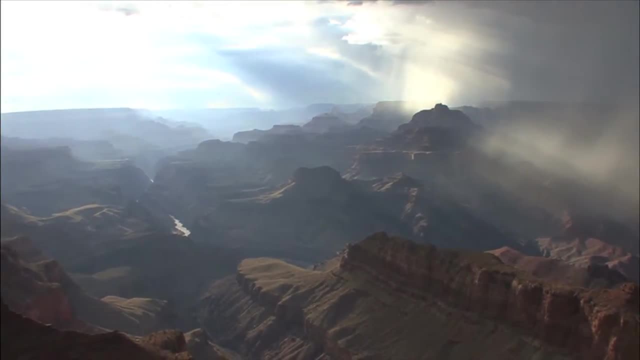 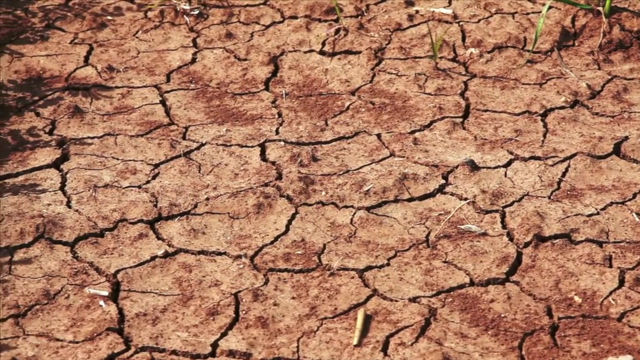 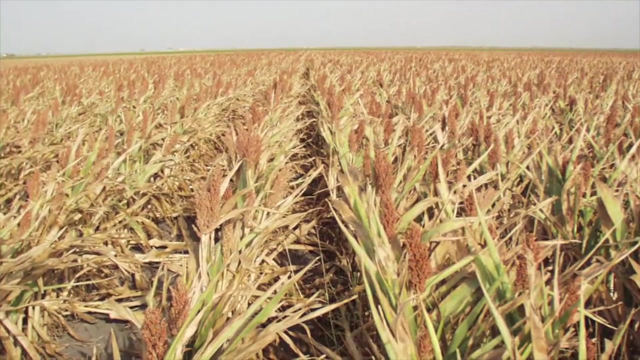 Sometimes places don't get enough rain. When this happens, there can be a drought. Drought is when you have less rainfall than you expected over several months or longer. Droughts can be dangerous, too For farmers. drought means that you do not have enough water. 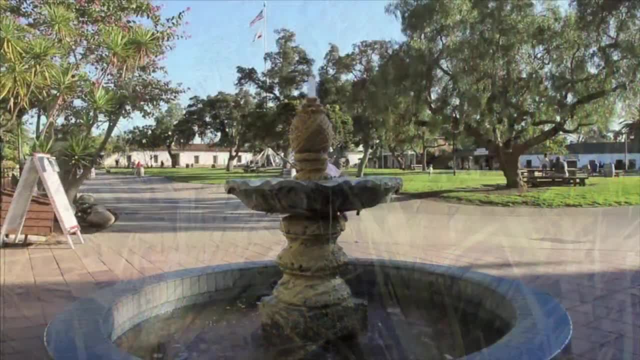 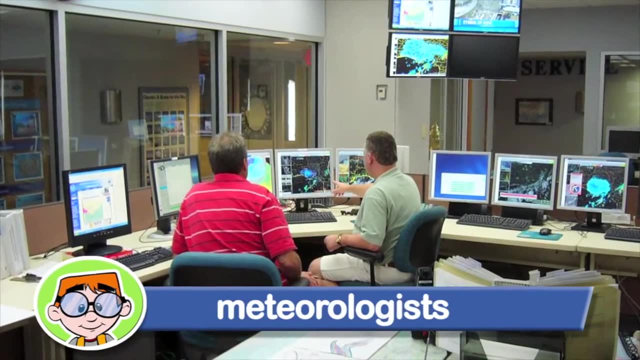 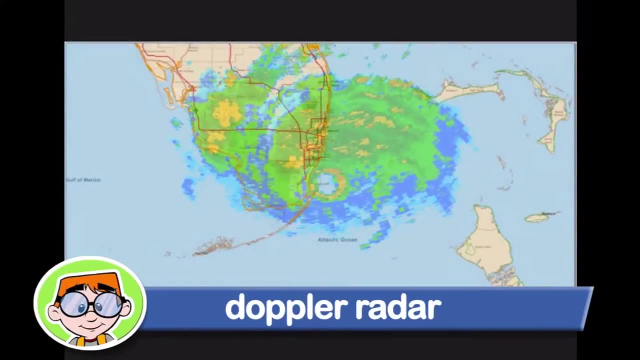 in the soil for crops to grow. In a city or town, people may be asked to conserve water. Today, meteorologists- the scientists who study weather, have tools like Doppler radar. Doppler radar can detect a rainstorm, its size, intensity and direction. 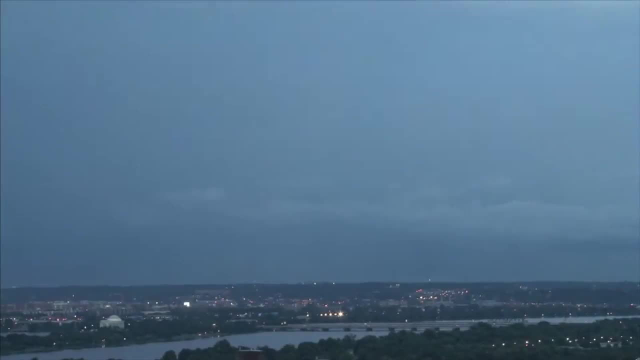 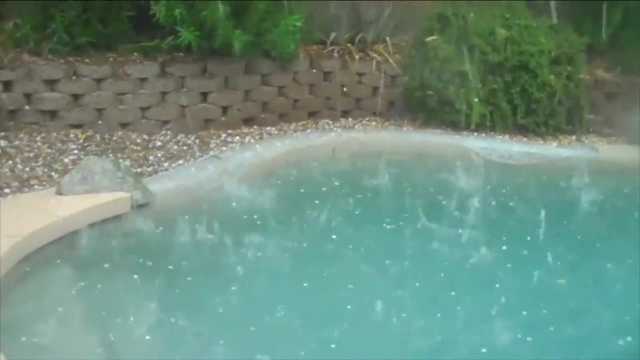 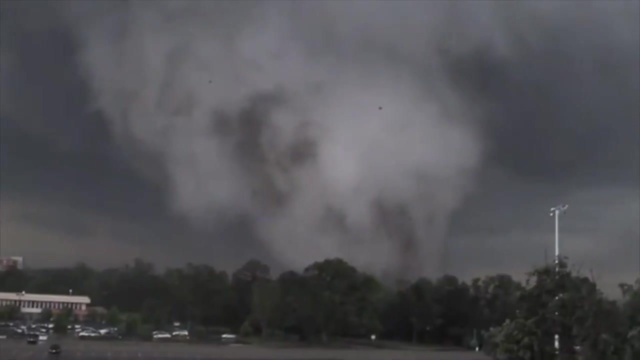 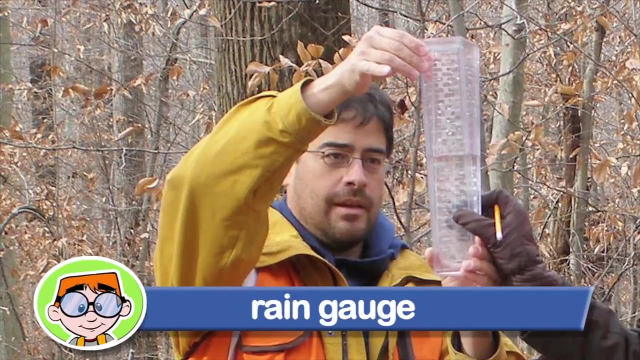 Because of Doppler radar, forecasters can warn people of severe thunderstorms that may bring strong damage, such as raging winds, large hail, heavy rain and possibly tornadoes. Meteorologists can also measure how much rain has fallen. They do that by using a tool called a rain gauge. 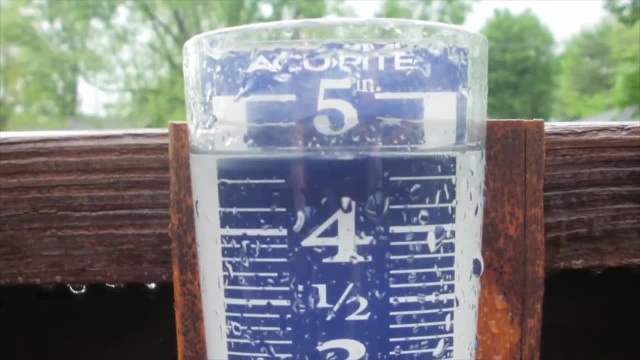 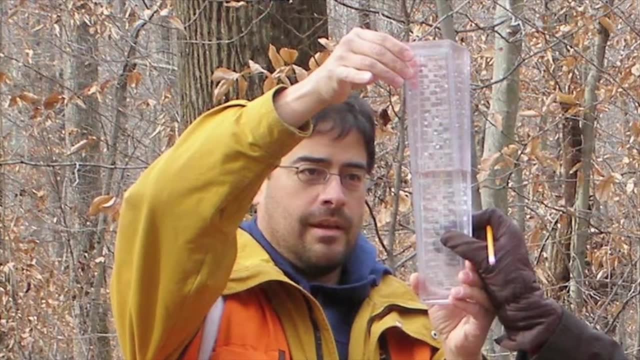 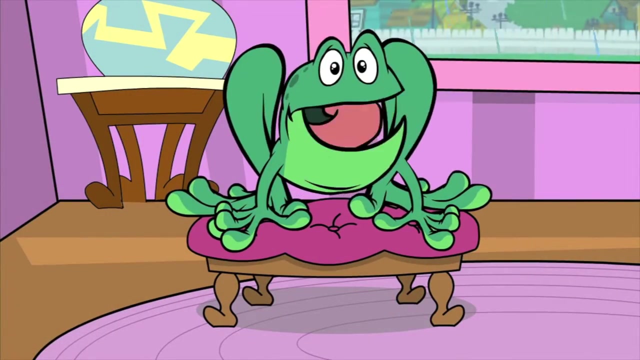 A rain gauge is a container, much like a bottle, that is left outside. It fills up with rainwater and the meteorologist then measures how much rain has fallen. So we all need rain, but too much or too little can be a problem. 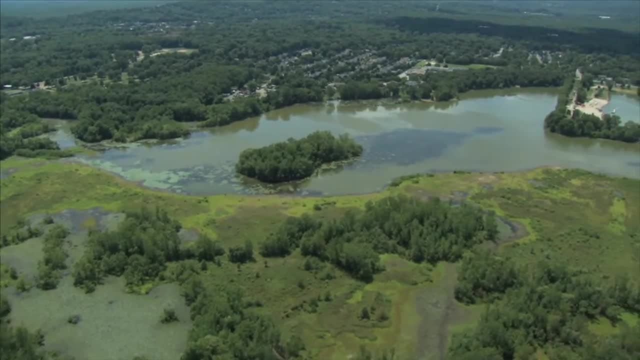 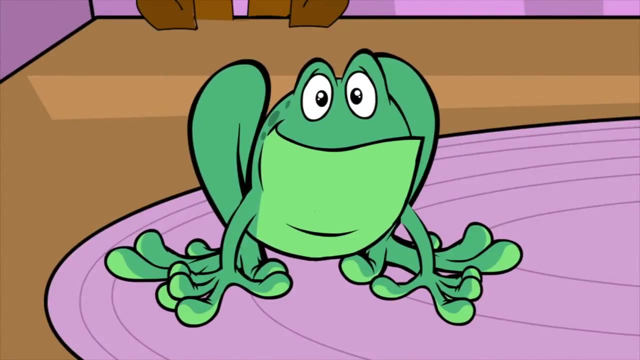 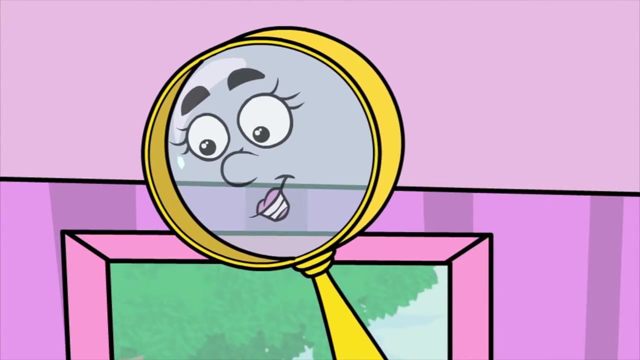 Exactly: Floods or droughts are both dangerous to people, animals and plants. Ah, I get it. Thanks, Maggie, You're very, very welcome. You're very, very welcome. You're very, very welcome. Today I learned a lot about rainstorms. 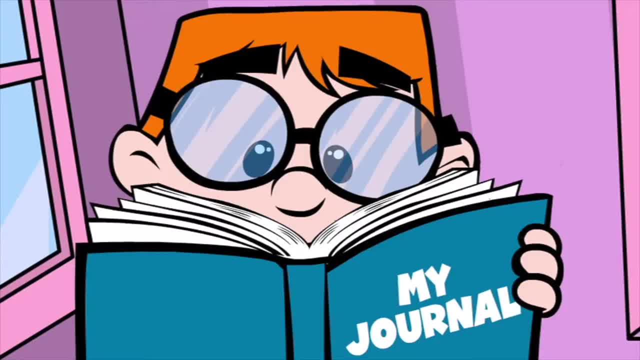 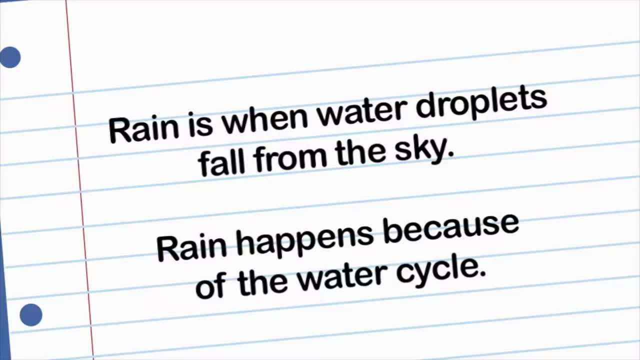 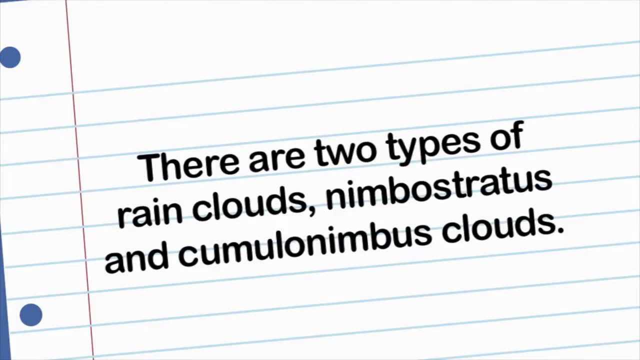 I hope you did too. These are the notes I took in my journal. Rain is when water droplets fall from the sky. Rain happens because of the water cycle. There are two types of rain clouds: nimbostratus and cumulonimbus clouds.